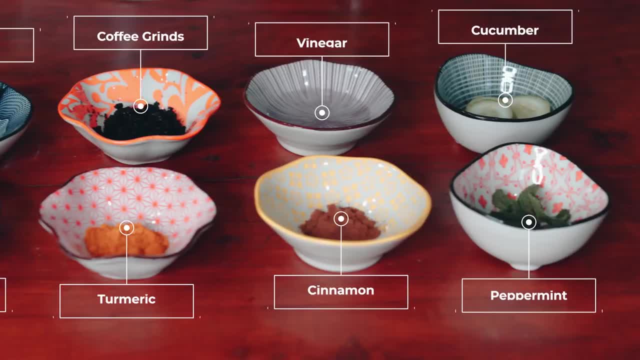 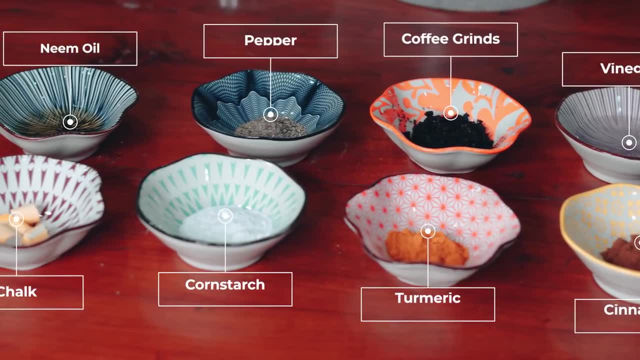 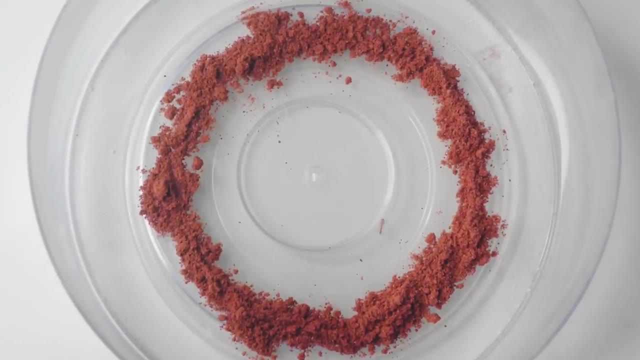 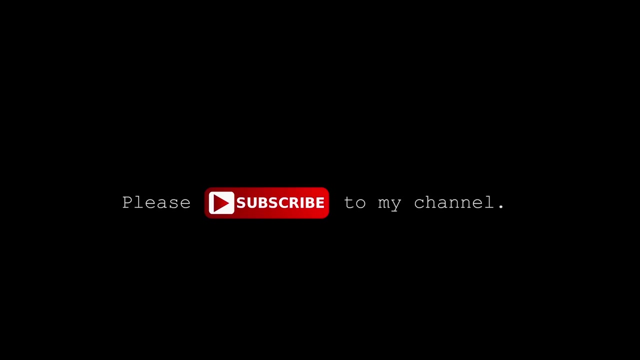 Which of these 10 natural, eco-friendly ingredients works best at repelling or killing pest ants in your home. Well, today we're going to find out in the ultimate anti-ant substance test. Welcome to the AntsCanada ant channel. Please SUBSCRIBE to my channel and hit the BELL icon. 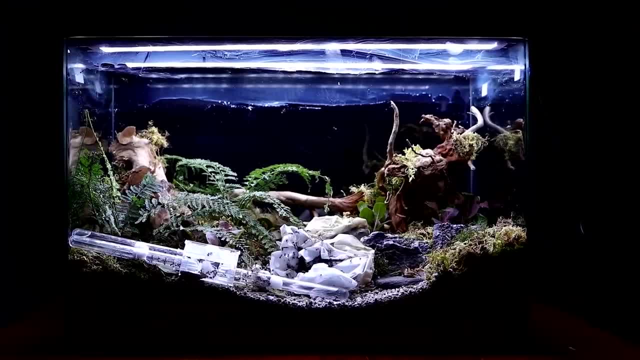 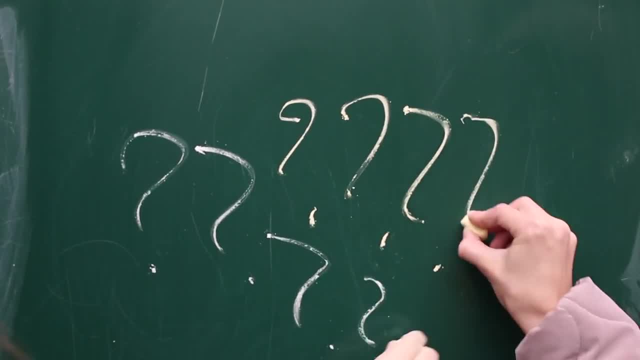 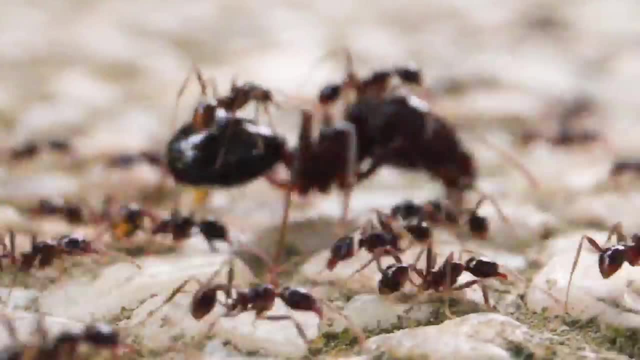 Welcome to the AC Family Enjoy. In all my years of ant keeping, there is one question I receive the most above all other questions, and it's this: how do I safely get rid of ants from my home in the most humane or eco-friendly way? Wouldn't knowing this be an awesome help and alternative to calling? 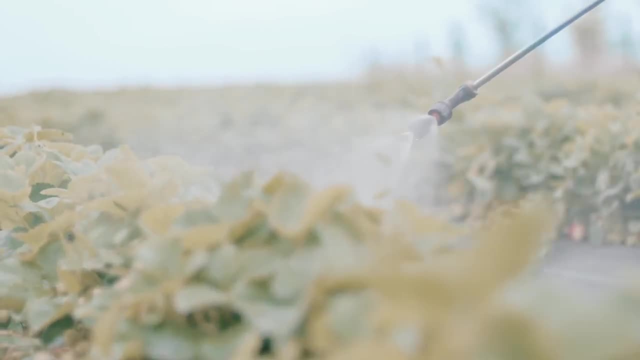 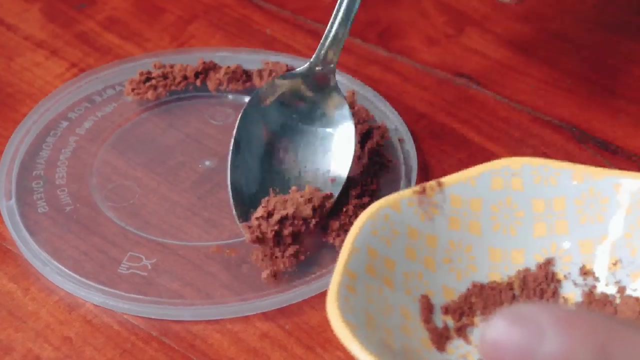 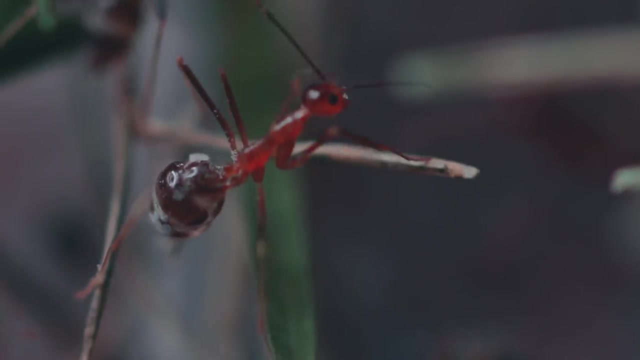 up a pest company, which will almost certainly resort to some kind of chemical to exterminate the ants, Which isn't the most eco-friendly method. So that's why this week I decided to conduct an experiment using live ants from an invasive yellow crazy ant colony I dug up from my yard as subjects for an ultimate anti-ant substance. 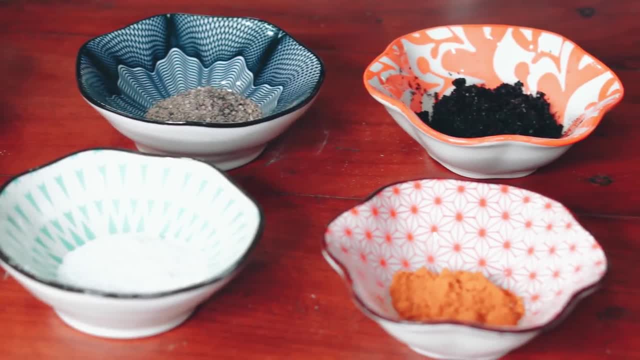 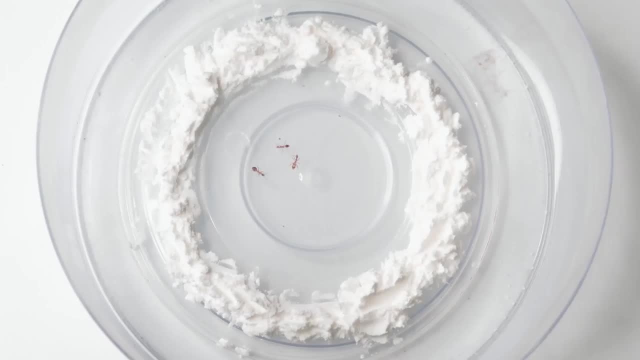 test using 10 natural items that are easy to find and are OK for the environment as well as safe for use around human homes. I'll tell you now. I was pretty surprised at some of the results, And I'm sure some of you might be too. 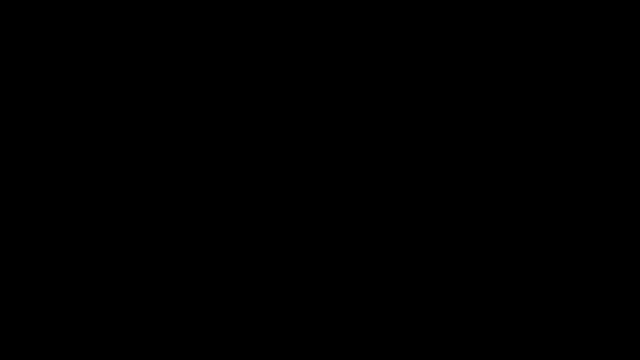 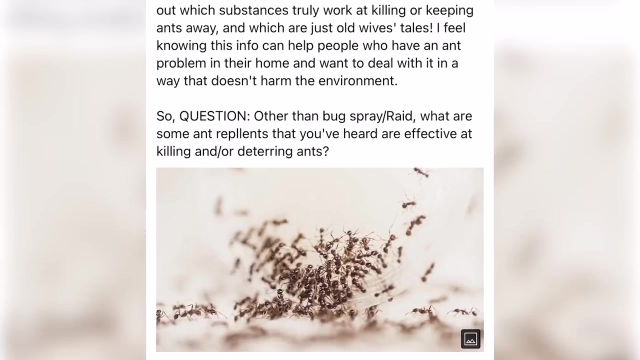 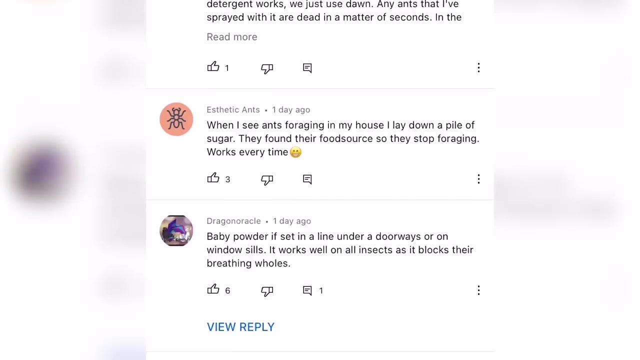 So keep on watching until the end. Now let's go over the The Anti-Ant Experiment. I asked you guys in a community tab post to list some home remedy type things you heard are good at repelling or killing ants, And from all your amazing and sometimes surprising suggestions, I chose the 10 most common ones. 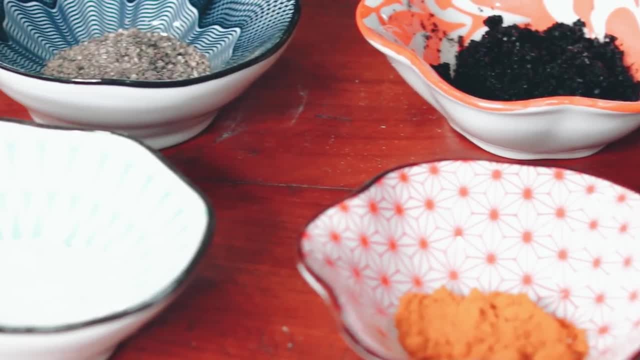 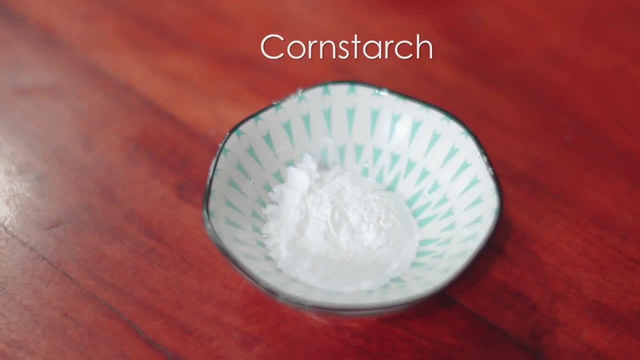 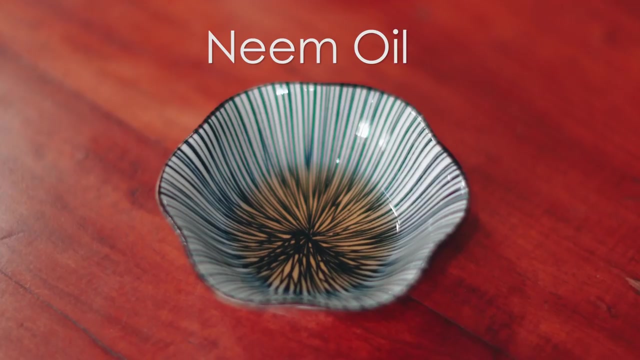 Here are the 10 items we will be testing for their ant repelling capabilities today, as suggested by you, the AC Family: Cinnamon, cucumber, cornstarch, peppermint, coffee grinds, vinegar, black pepper, turmeric, neem oil and diatomaceous chalk. Now to test each of these items, I will be using this. 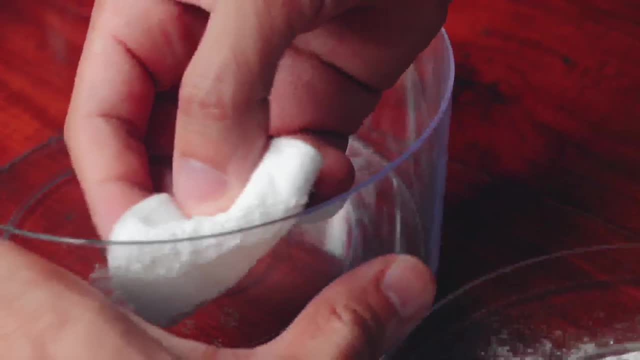 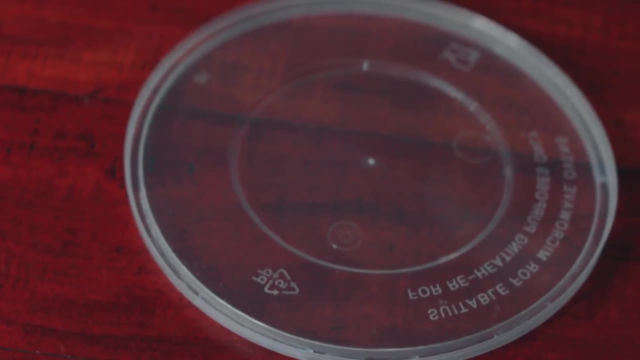 round container. I'll need to place baby powder on the inside of it to keep the ants from crawling out during the experiment. I'll also be needing this smaller plastic lid as the base for each substance, which will make it easier to swap out and not leave any traces of substance behind. 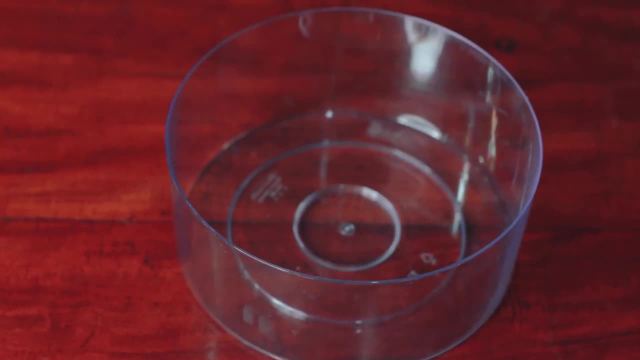 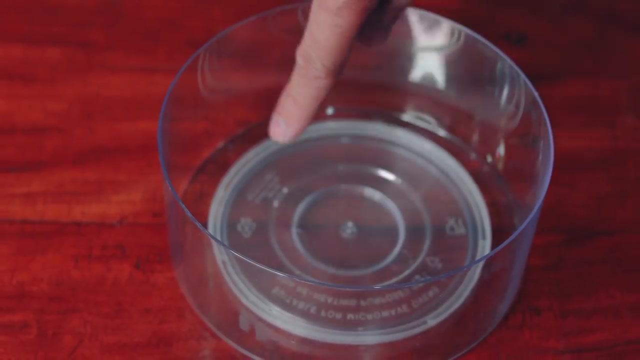 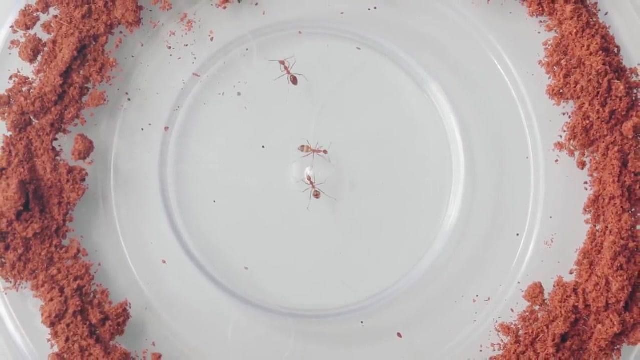 for the most accurate results. The way it'll work is using each substance one by one. I will create a ring on the lid, then place in three ant workers into that ring. Once inside the ring, the ants will instinctually panic being in a foreign area and will automatically try to. 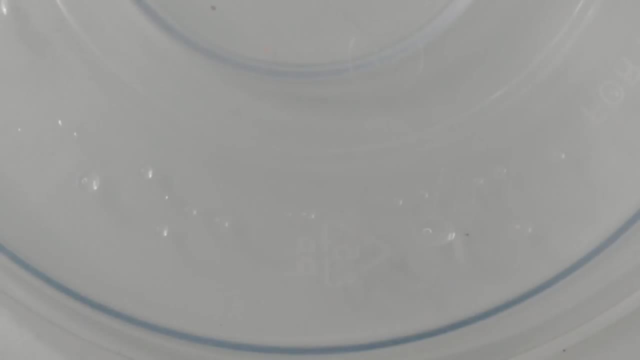 find their way back home to their colony and, in doing so, will be compelled to cross over to the other side of the container. Once inside the container, the ants will automatically try to find their way back home to their colony and, in doing so, will be compelled to cross over to the 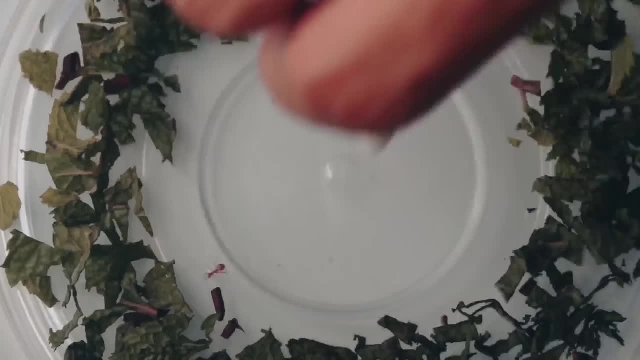 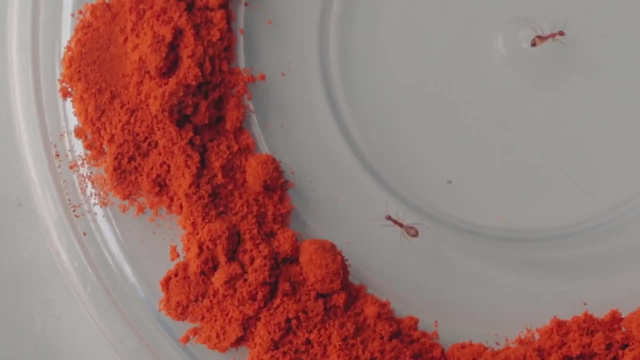 other side of the container and, in doing so, will be compelled to cross over to the outside of the ring. However, if the substance is truly an effective ant repellent, the ants will choose to not cross the ring and instead remain inside the circle or even die after crossing it. If the substance 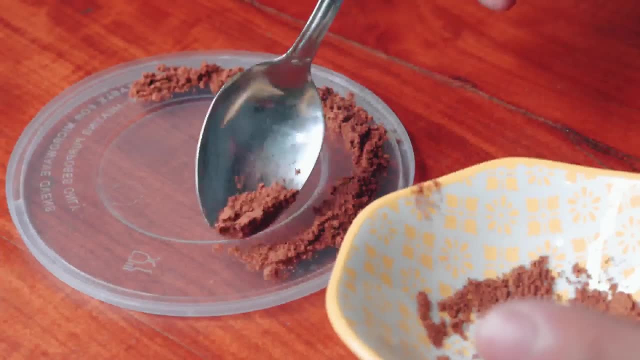 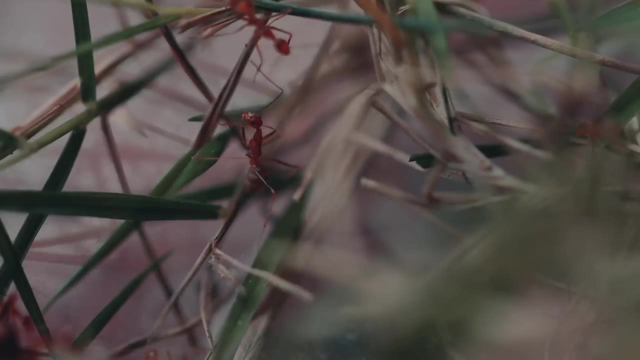 isn't an effective ant repellent, the ants will simply cross the ring unharmed. Sounds easy and straightforward, right? Well, AC Family, there's a bit more. Here is the yellow crazy ant colony collected from my yard. As an ant lover, I 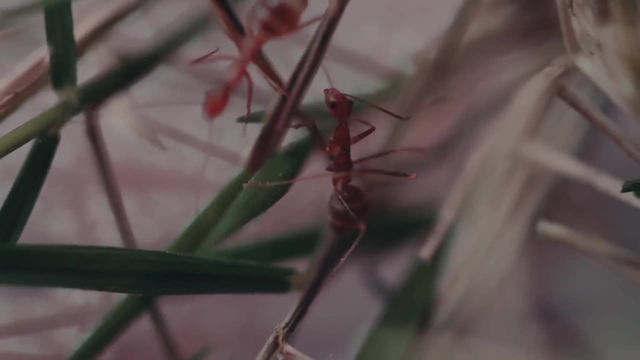 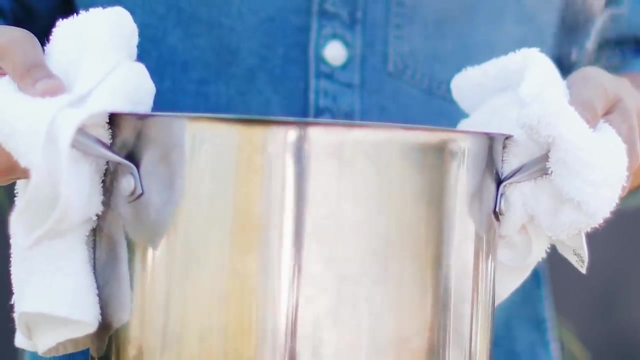 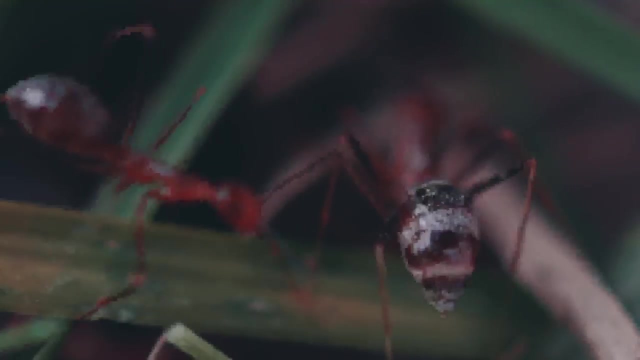 usually don't enjoy killing ants, but if you've been watching this channel for a while, we are on a mission to get rid of these invasive ant species to help protect the native ones living in my yard and the entire ecosystem of my area as a whole. So I felt these yellow crazy ants would make. 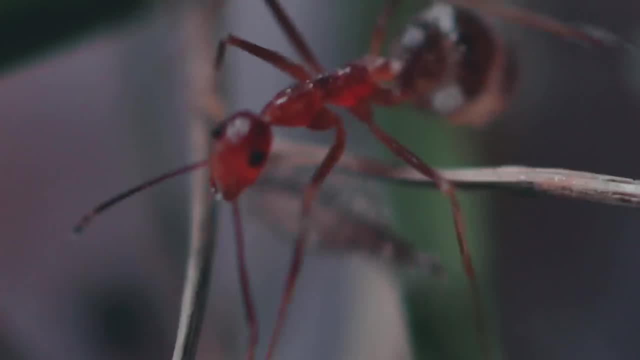 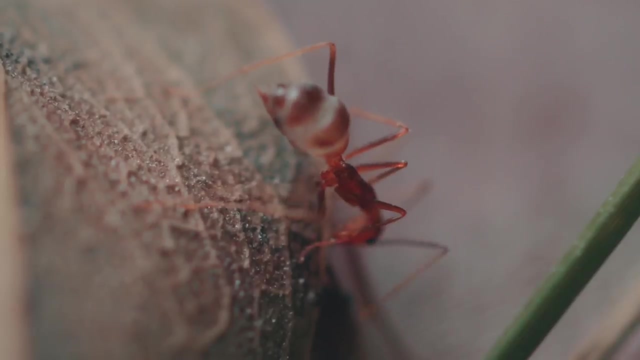 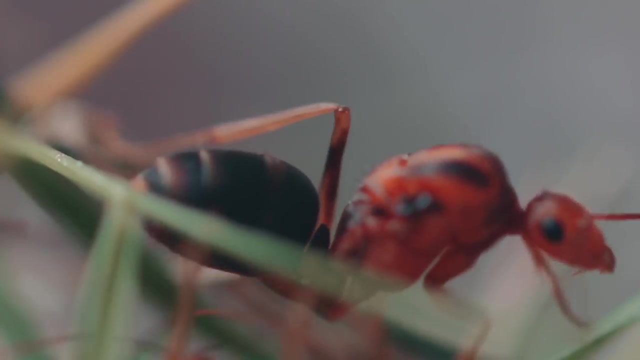 suitable test subjects, because if they end up dying, then that's OK and their deaths won't be in vain, as they will help contribute to science. But guys, check this out: Inside this colony, I managed to collect several queen ants as well, So I decided that I could also. 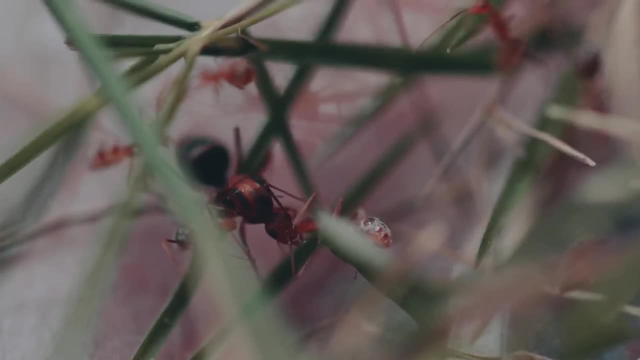 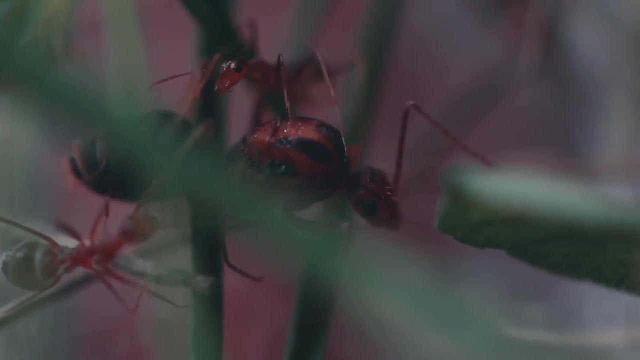 test the effectiveness of the ant repellents on the queens whom, if you're really trying to get rid of an ant colony from your home, is the one you truly want, dead or gone, because she's the one giving birth to all the ants in the first place. 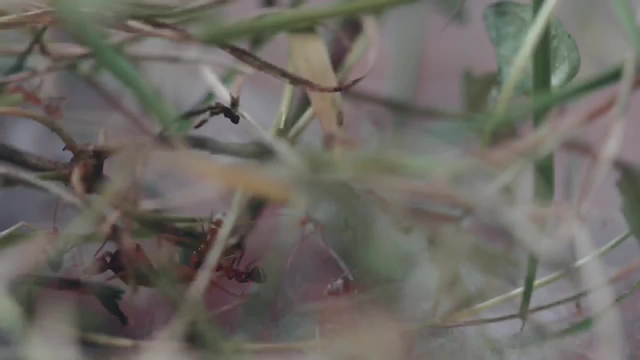 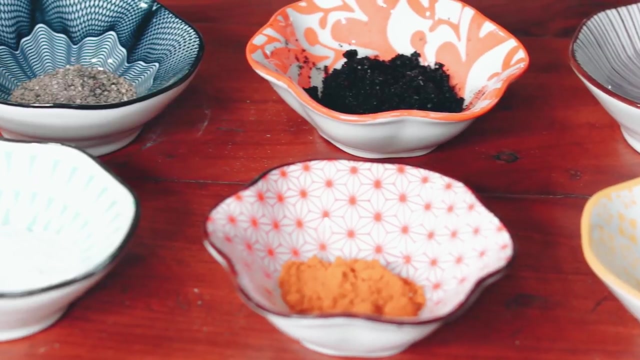 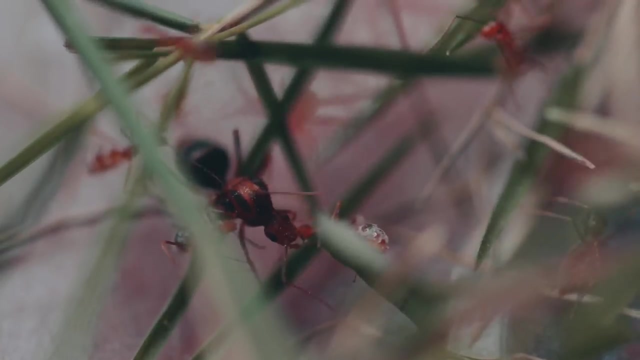 essentially the source of every ant home infestation. So stay tuned for the bonus anti-queen on the items we find to be the most effective on the worker ants to be held towards the end of the video, Without any spoilers, the results on which substances repel and or kill the queens. 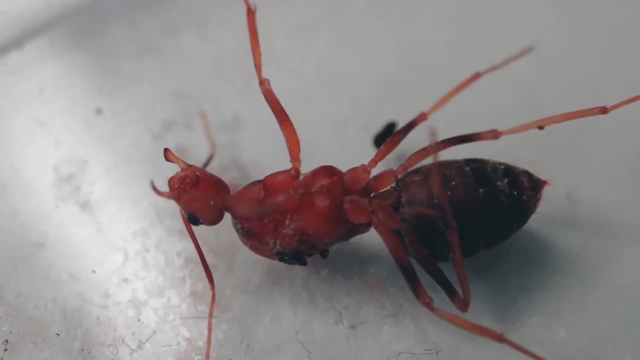 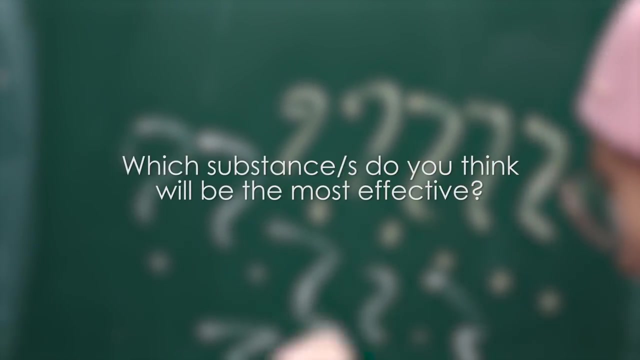 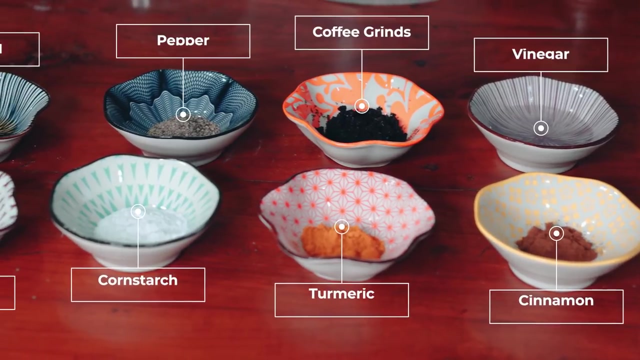 may actually surprise you. Sound like a plan, guys. So what's your hypothesis? Which substance or substances do you think will be the most effective at repelling or killing ants? Let us know in the comments section and at the end, go back to your comment and see if you were right. 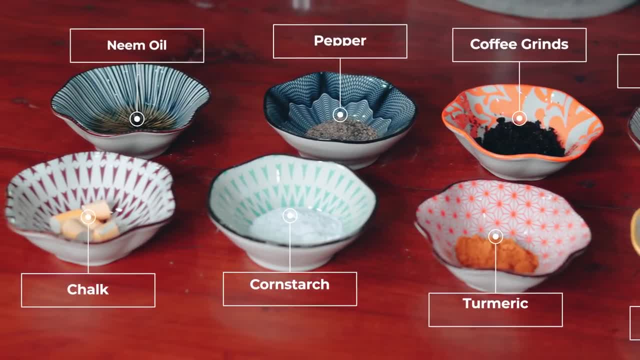 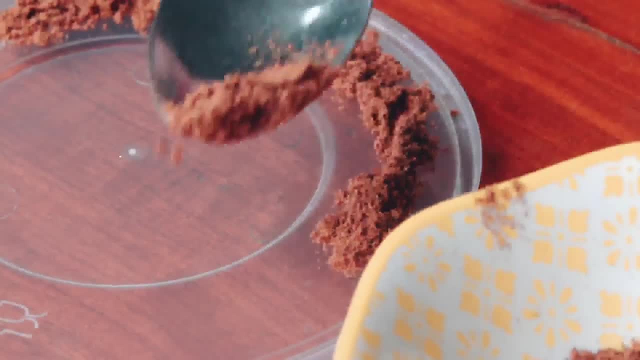 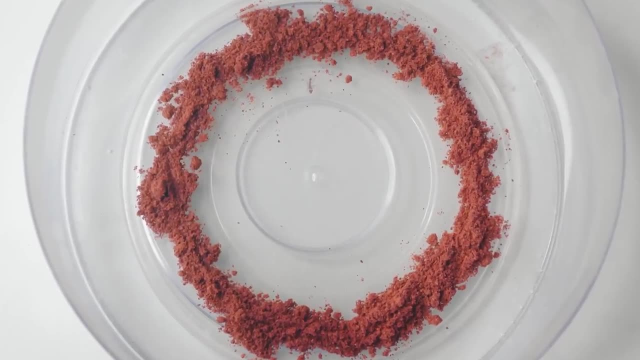 No cheating Guys. let the anti-ant experiment begin. First up is cinnamon. I formed a cinnamon ring onto the platform, then placed the whole platform inside. The stage was set. I then grabbed a worker ant from the colony and placed it inside, along with two other workers- AC Family. let's watch. 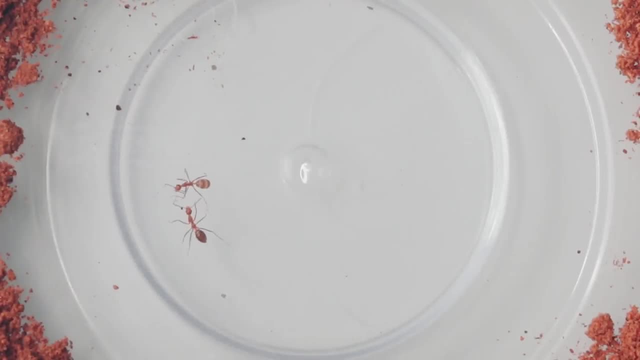 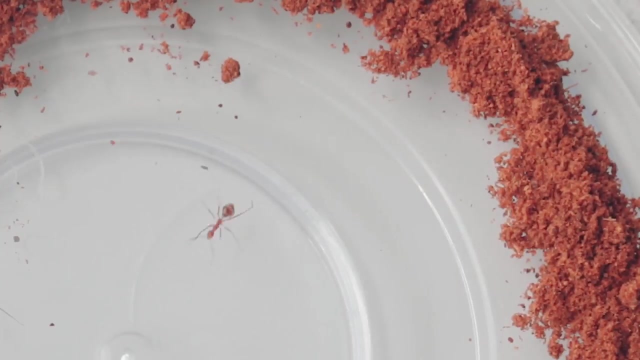 At first the ants wandered around and indeed seemed to avoid crossing the cinnamon ring. Wow, The ants scurried all around, trying all points of possible exit from the ring, But it did seem all three worker ants did not want to cross the cinnamon. 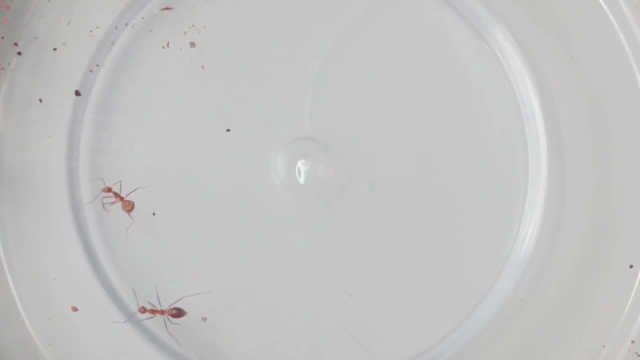 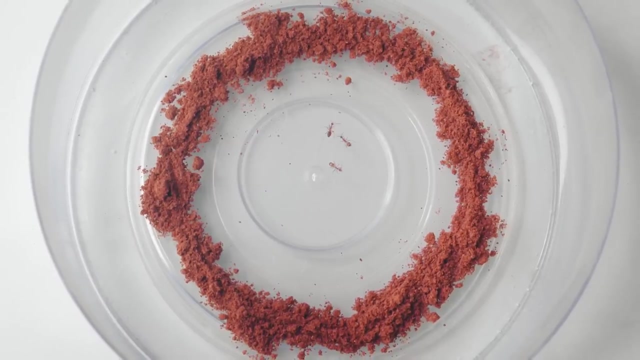 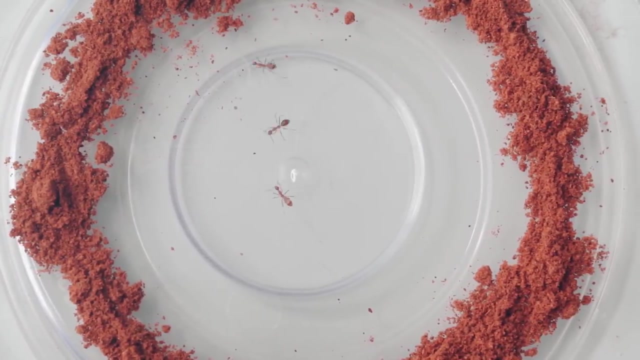 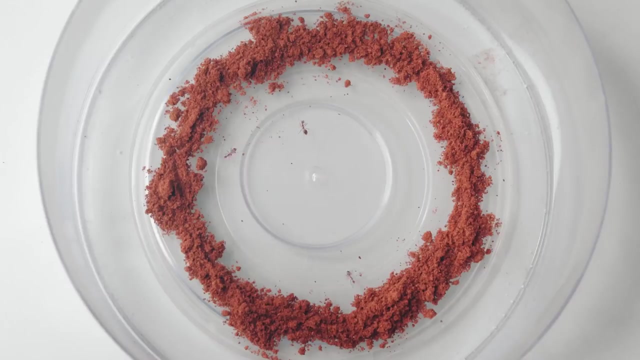 Let's give them a few minutes, guys, and watch what happens. Turns out they didn't want to cross the cinnamon ring. Turns out, almost ten minutes later the ants were still not willing to cross the cinnamon. So AC Family, this tells us that cinnamon is indeed a good ant repellent. We'll be testing. 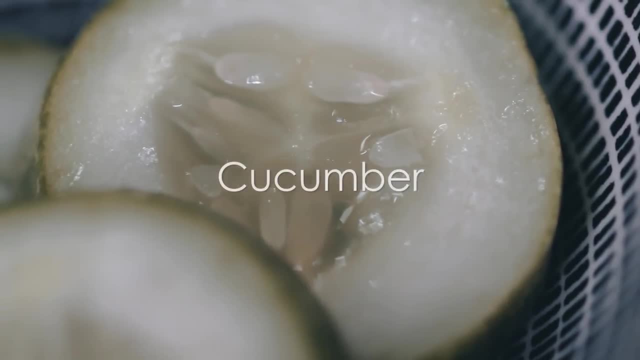 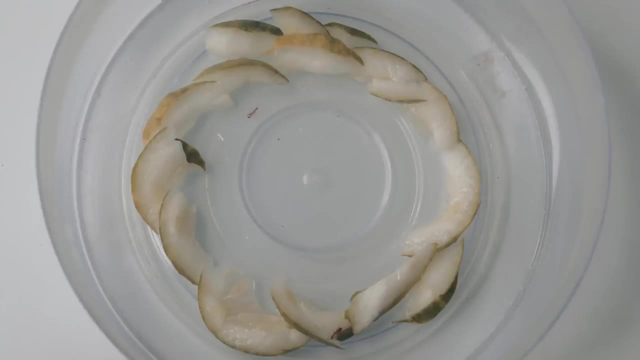 this on a queen. later, Next up, cucumber. I placed in the ants, but before I could even get the third ant in one of the first, two ants already were crossing the cucumber ring. Eventually, all three ants crossed the cucumber ring unfazed and unharmed, Turns out, cucumber is. 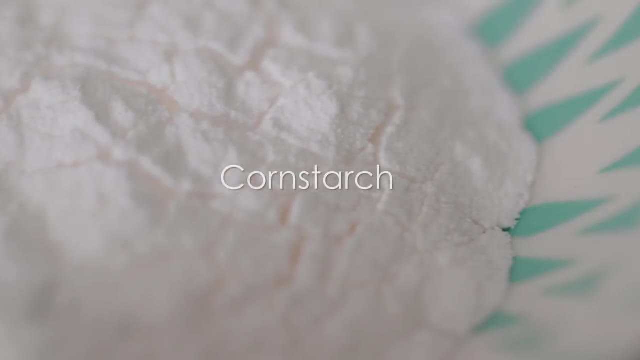 not an effective ant repellent. Next, we test cornstarch. A lot of you mentioned this option and I couldn't wait to see if it would work. At first, the ants seemed to want to avoid crossing the cornstarch ring. 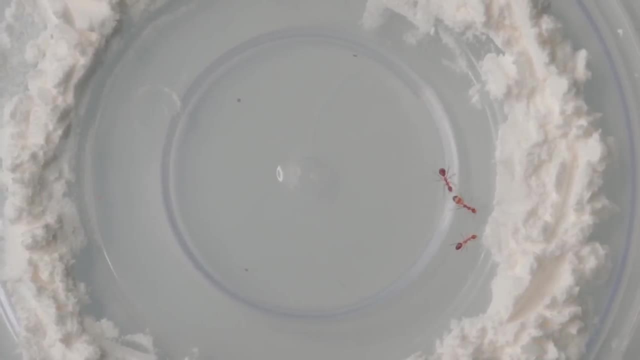 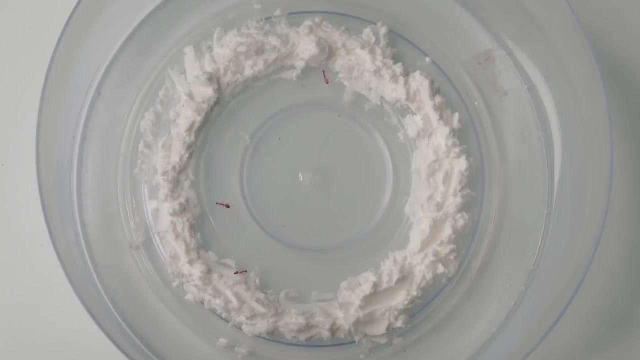 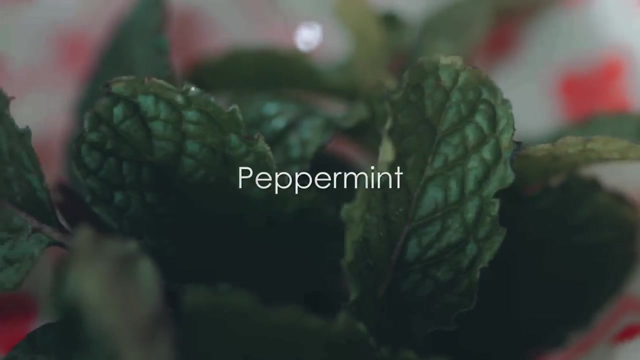 Could this be as effective as cinnamon was? Nope, An ant eventually crossed over it a few times and eventually made it unharmed. to the other side, Cornstarch is not an effective ant repellent either. Next up, fresh peppermint leaves I placed in the ants. 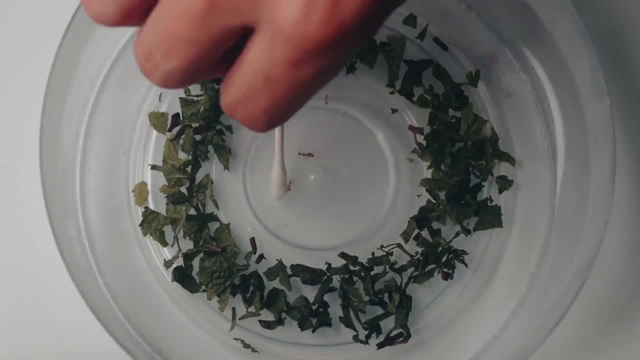 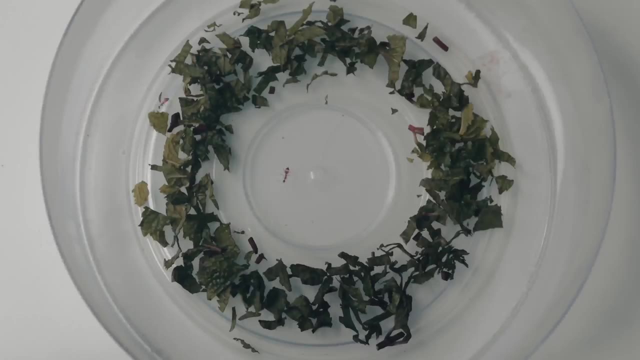 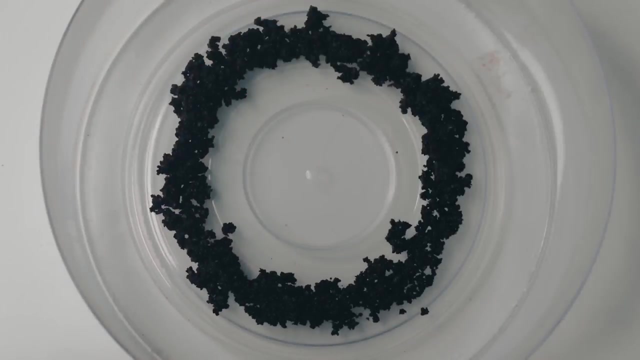 and the ants right away seemed OK with walking on top of the peppermint leaves but not crossing it. Then eventually an ant did cross over. so turns out peppermint was also not an effective ant repellent. OK, let's try coffee grinds. Maybe the caffeine turns the ants off. 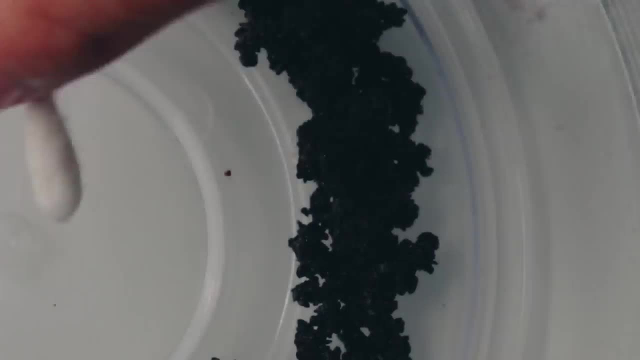 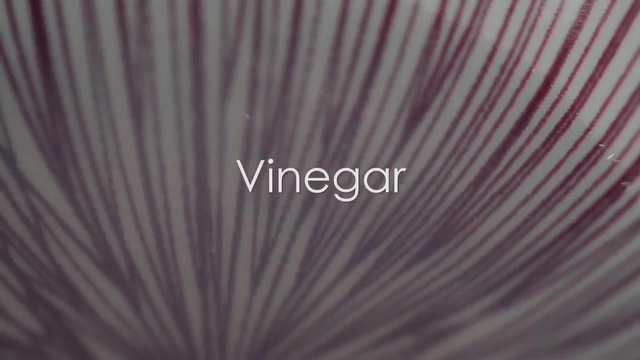 Uh nope, They crawled over the coffee ring pretty quick. Hey, I don't blame them. Fellow coffee addicts, raise your hands, Man will vinegar work. I know this is great at wiping out ant pheromone trails, but were they good ant repellents? 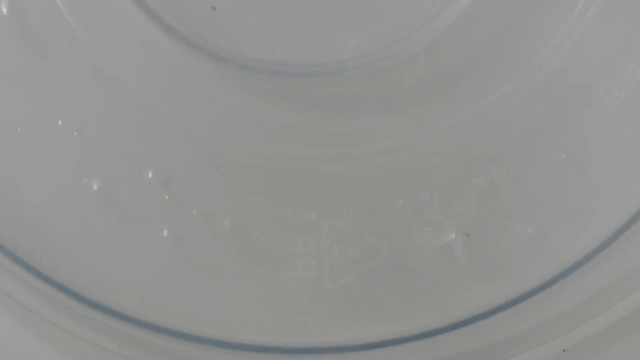 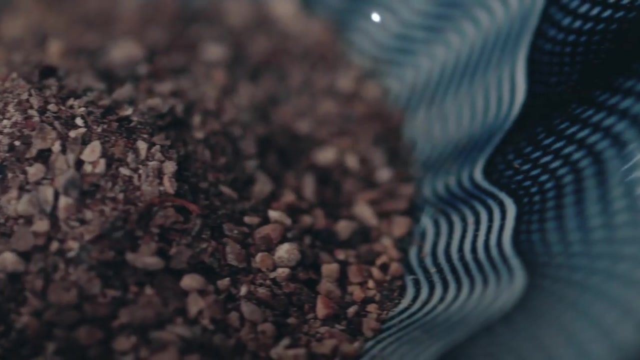 I placed in the ants. and sure enough, the ants crossed the ring and wandered to the outside. Vinegar is not an effective ant repellent either. How about black pepper? Perhaps it would be too spicy for the ants to cross? I placed in the ants. 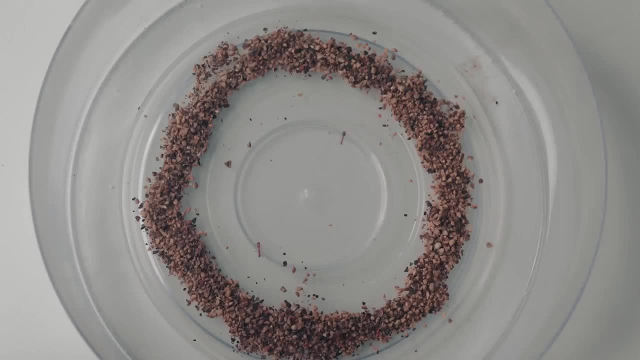 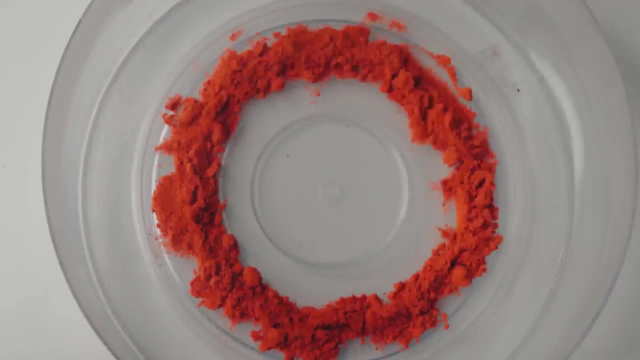 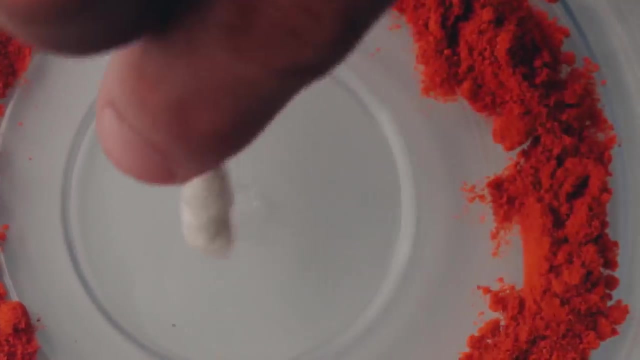 but nope, Seems the ants were unharmed, Unphased by spice, not an effective ant repellent. Let's test turmeric. Surely this strong spice will turn the ants away or kill them. I placed in the ants. At first it did look like the ants were avoiding the turmeric. 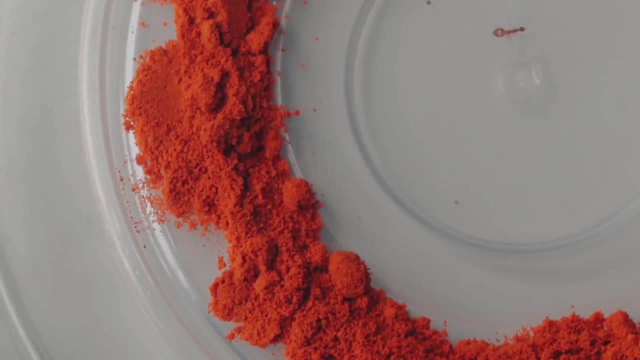 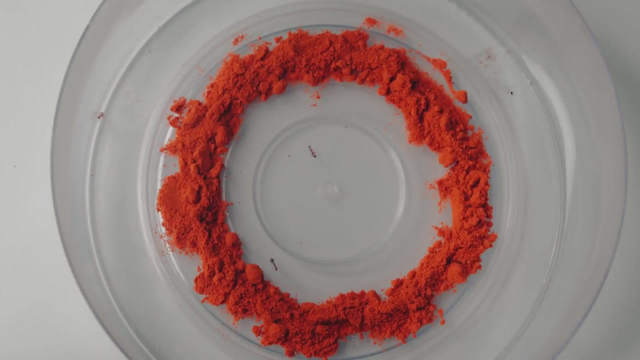 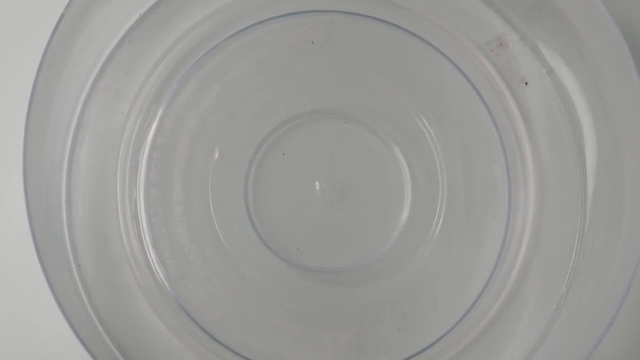 just as they did the cinnamon, but in no time an ant crossed over unharmed. Turmeric is also not an effective ant repellent. Just two more left. Neem oil Now. this potent stuff is a great antifungal and, I heard, anti-mosquito, but does it work against ants? 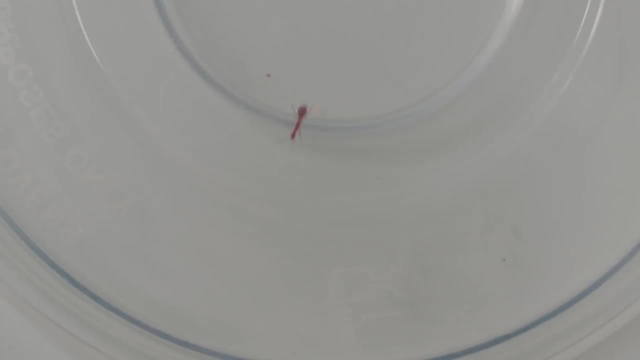 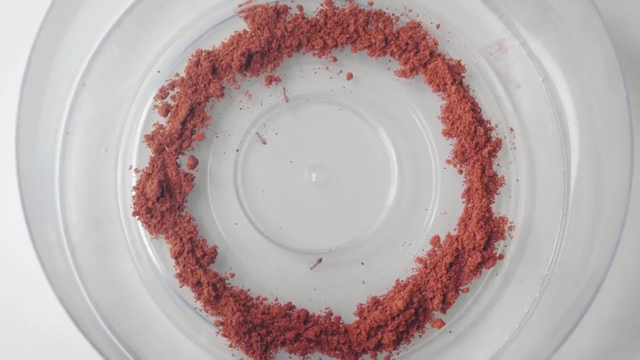 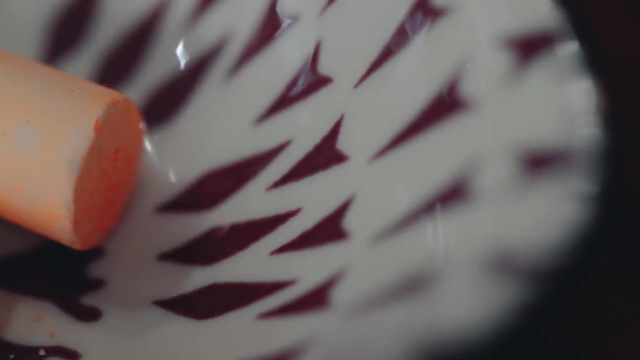 I placed in the ants. Turns out, they too crossed over unharmed and unbothered. Wow, so far, none of these items, except cinnamon, worked at repelling the ants and none killed them. But now we come to this stuff. Last but not least, we come to diatomaceous chalk. This is a substance 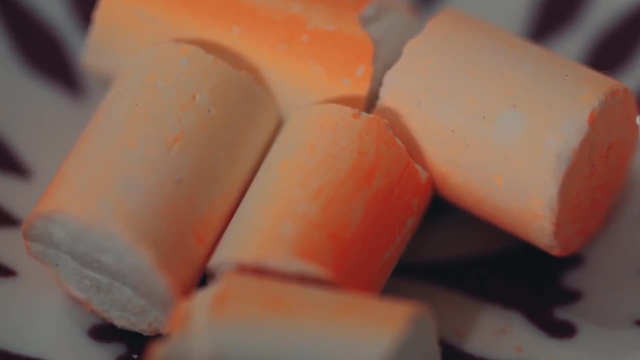 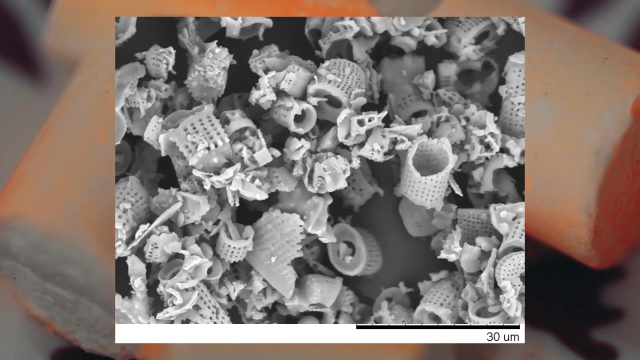 that is well known to kill nearly all the plants. It is a substance that is well known to kill nearly all insects. It's essentially a chalk made of fossilized marine microbes called diatoms that stick on to an insect's exoskeleton- And well, I won't spoil it. Just watch what. 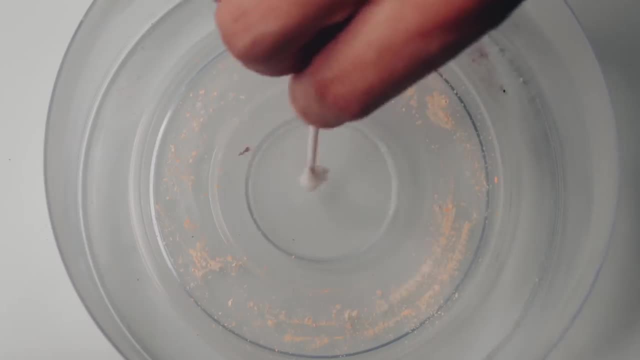 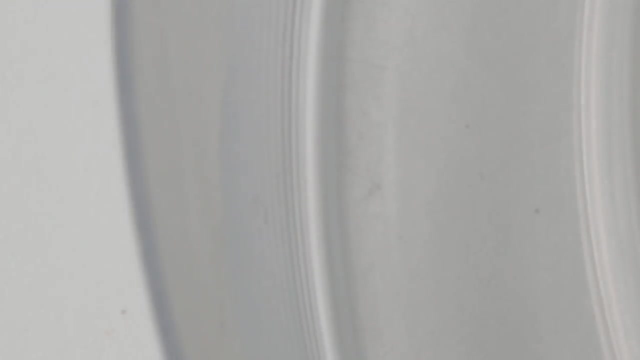 happens when I place the ants in. I placed in three ants and eventually they all crossed over to the other side, seemingly unfazed and unharmed, But AC Family. what I saw next was truly difficult to watch. It quickly became apparent that the ants' walking capabilities 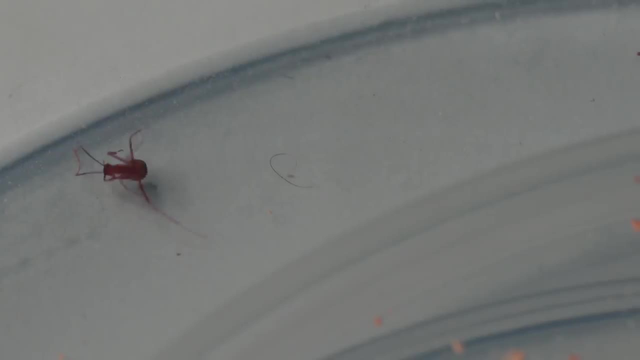 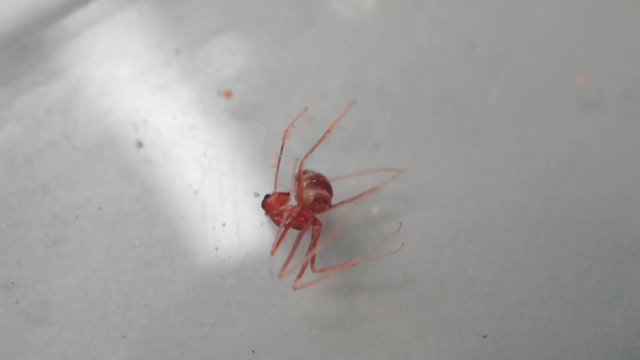 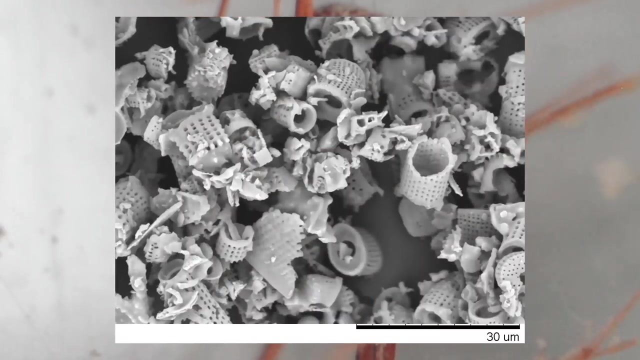 were being hindered. and then one ant suddenly began to coil and convulse. It began to die a quick but painful-looking death. So what you're seeing here is the aftereffect of crossing this diatomaceous chalk: The fossilized diatoms stick to the exoskeleton of the ant, creating 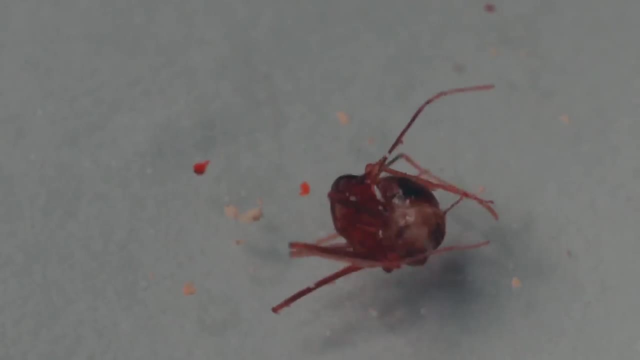 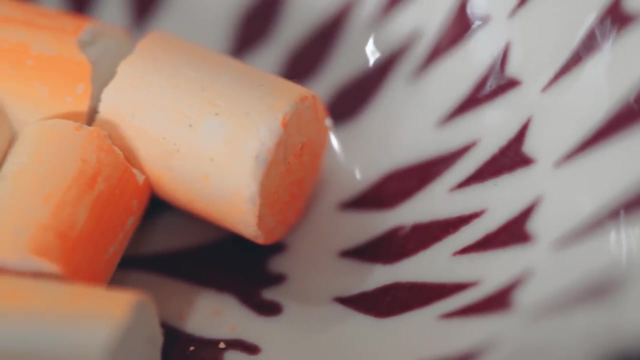 a tonne of microscopic cuts, which essentially causes the ant to get stuck on the ground. This diatomaceous chalk or earth is lethal to insects but safe for humans. In fact it's so safe it's placed into cereals, breads and grain products to help reduce the infestation. 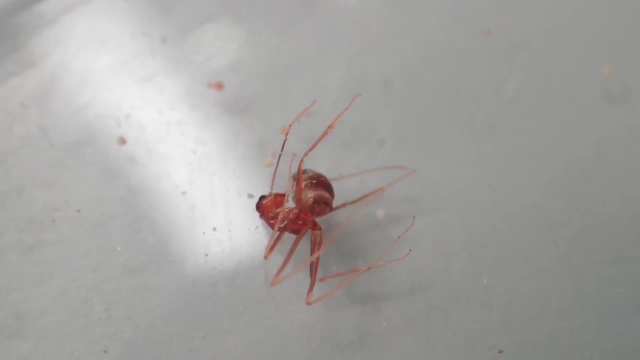 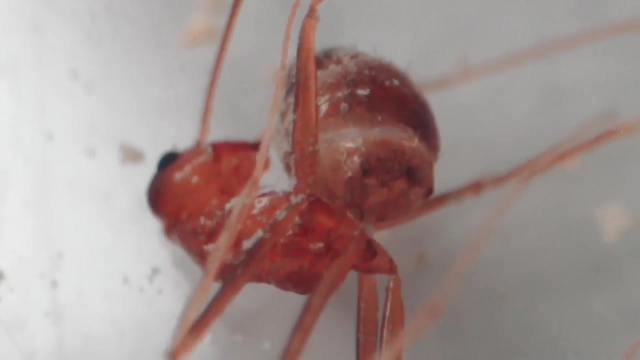 of grain-loving insects. It was sad to see the ants die, but at least we had recorded and proven that indeed, this diatomaceous chalk was lethal to humans. Indeed, this diatomaceous chalk was not just an effective ant repellent, but an effective 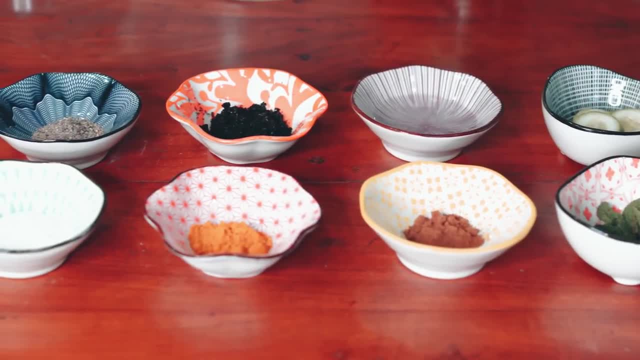 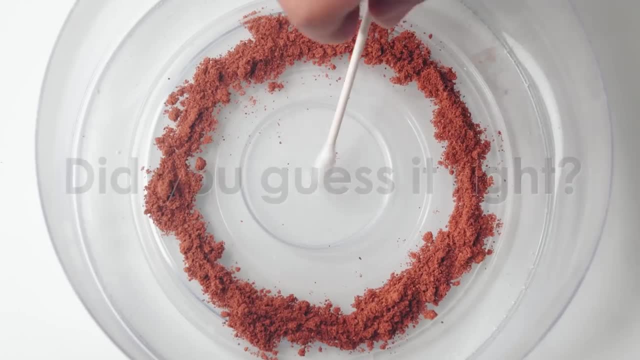 ant killer. And that was it. After testing all items, turns out only cinnamon and diatomaceous chalk actually worked against the worker ants. Did any of you guess these correctly? In other words, did these results surprise you? Think about it. 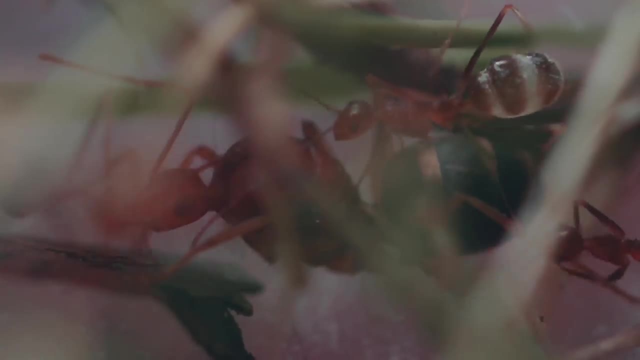 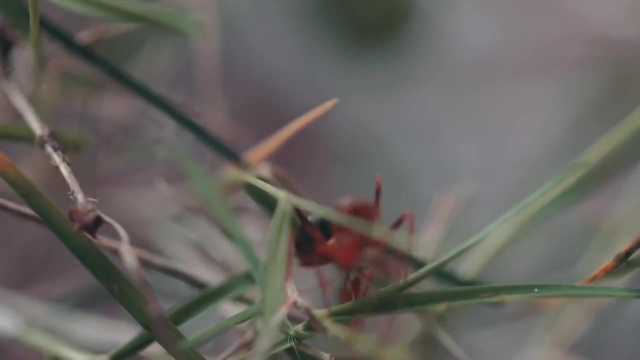 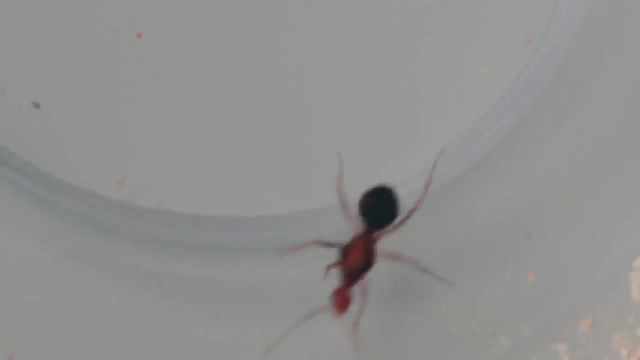 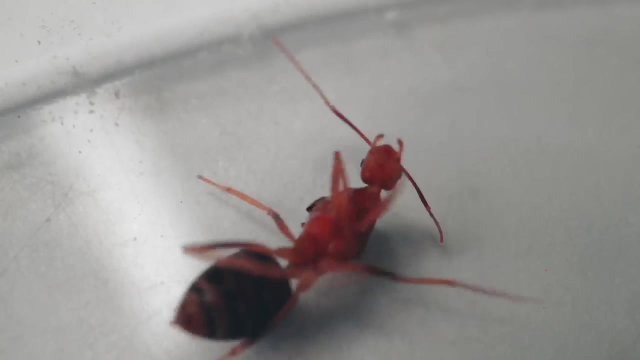 And as for diatomaceous chalk I placed in the queen ant, she crossed over the ring and, just like the workers, at first she seemed ok, But it wasn't long before she too began to show signs of death by fossilized diatoms. 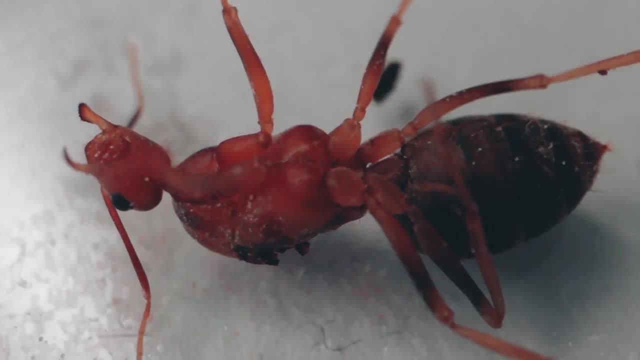 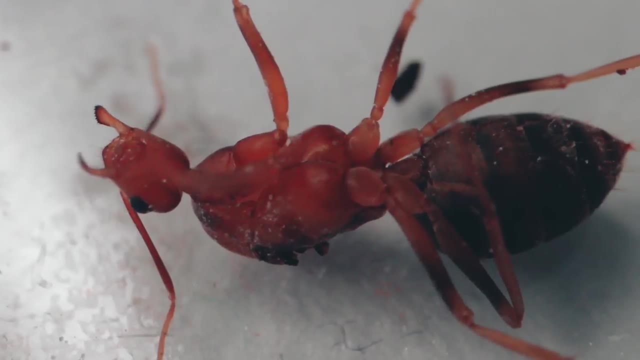 It was again sad to watch the queen die like this, but again, this needed to be done for the sake of the ecosystem of my area and was all in the name of science. So sorry, queen ant, thank you for giving up your life in order for us to learn. 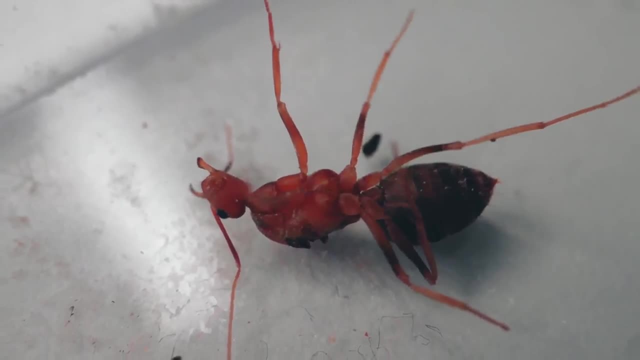 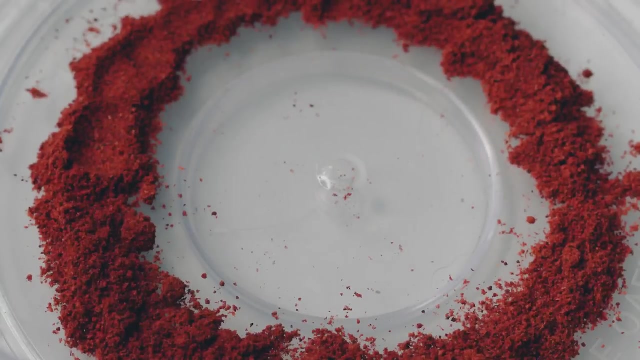 And so that was it, AC Family. In conclusion, we learned today that although cinnamon doesn't kill ants, it works at repelling worker ants, But not the queen. To be honest, this actually surprised me, because I always thought the cinnamon thing repelling. 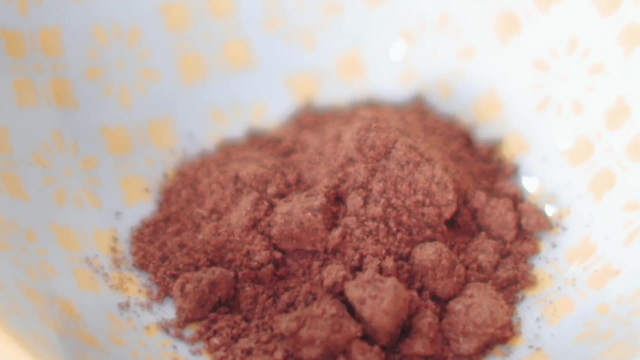 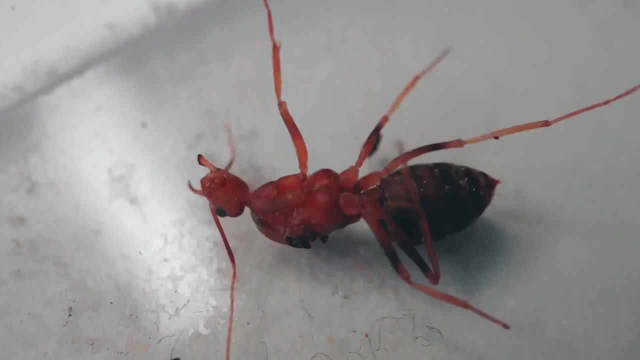 ants was a myth. Guess, grandmas the world over were actually right. As for diatomaceous chalk, it works effectively at killing both worker ants and queen ants. In terms of practicality, however, I feel diatomaceous chalk to be the most desirable. 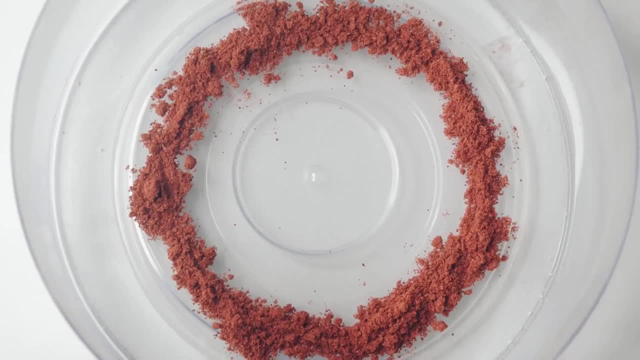 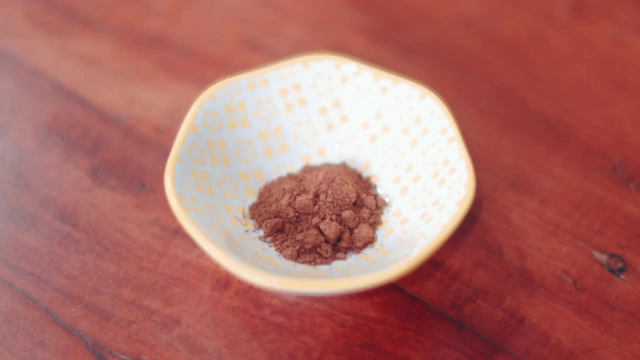 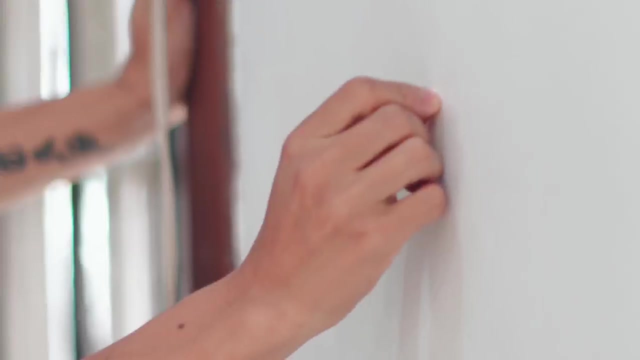 option for use at eliminating an ant problem. because what are you going to be creating rings of cinnamon all around your home? Though it might make your home smell real nice, I don't think your mom or dad would agree with this Chalk. however, drawn along the edges of a room, wall or floor might be more inconspicuous. 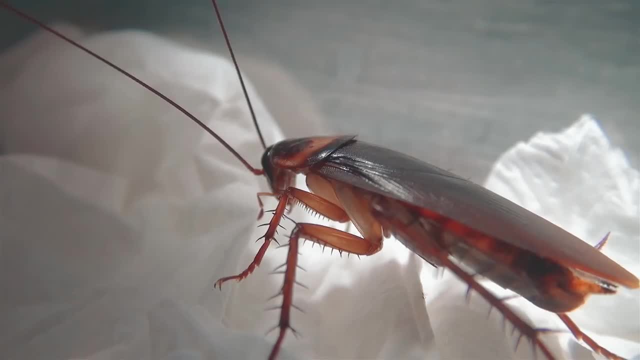 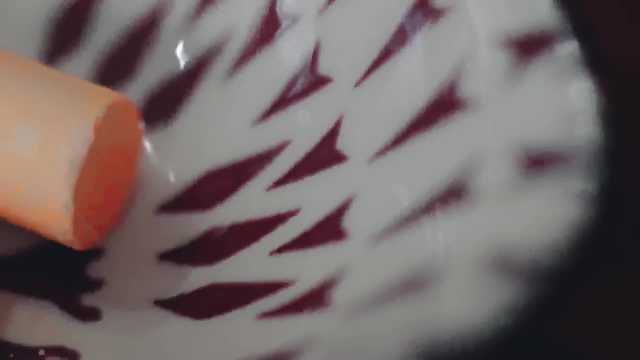 and easier to hide. I have found that chalk also works well with roaches and other arthropod pests, but you should note that it does become ineffective once it gets wet, and it eventually loses its effectiveness over time, So it must constantly be replaced. 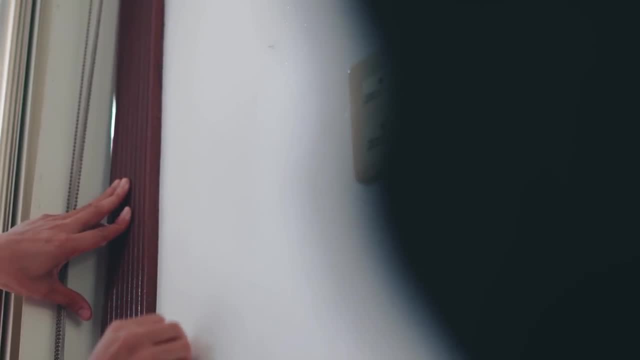 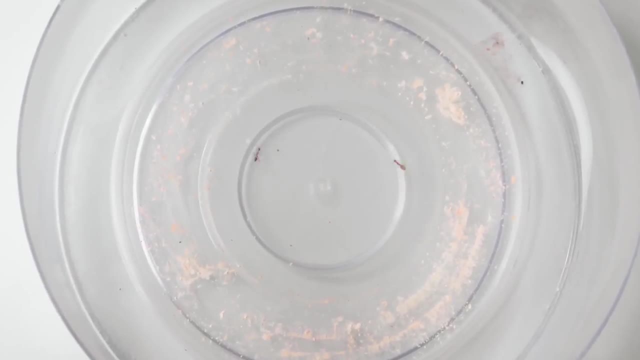 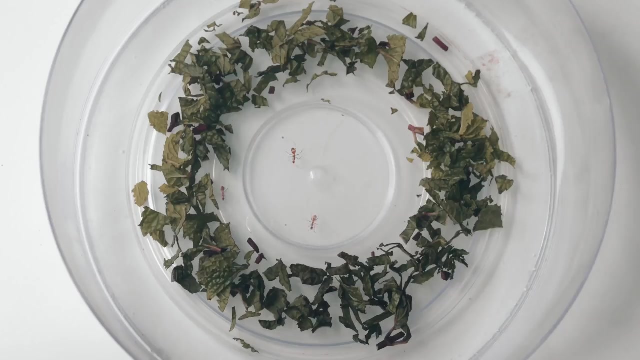 It should also be considered that, although cinnamon and diatomaceous chalk worked against these yellow crazy ants, it is still possible that they might not work on other species of ants, and perhaps some of these other items that we found don't work may actually be. 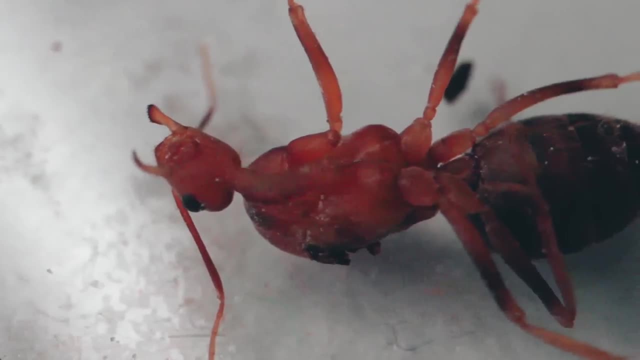 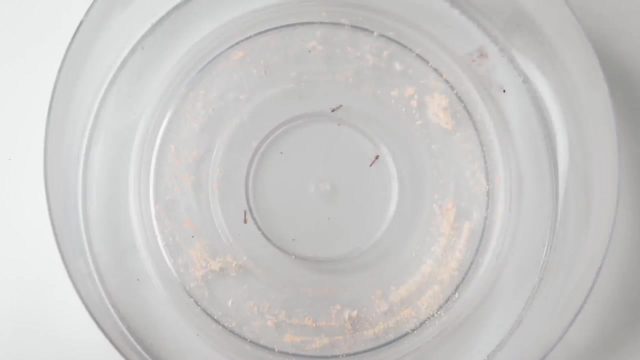 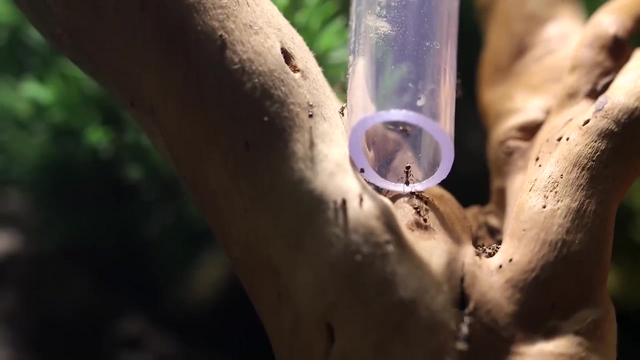 effective against other ant species But AC Family. overall, it was great that we learned and saw what we did today, because now we know the truth and can tell the world. Thanks for watching. I do understand that a lot of people do actually love ants but at the same time don't want. 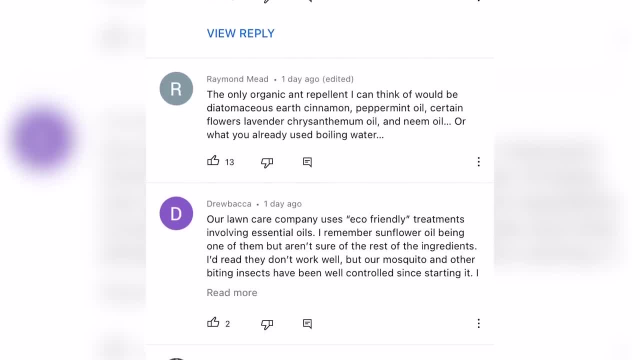 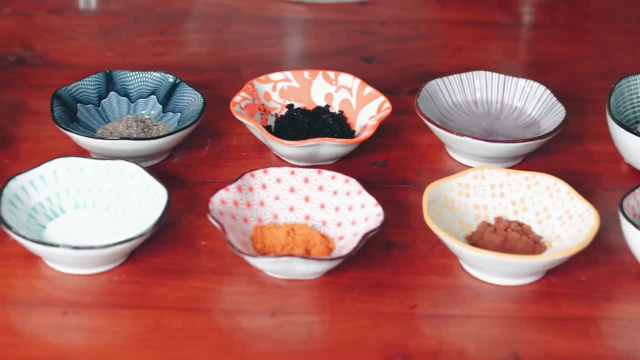 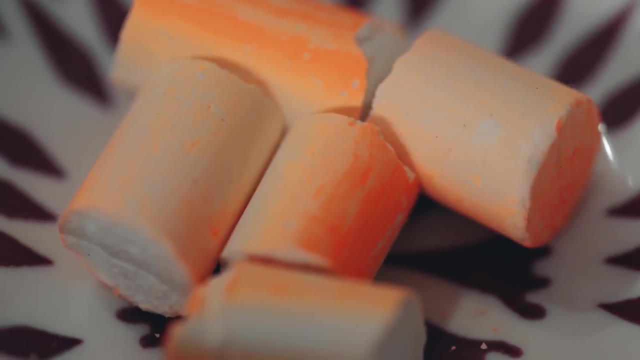 them wandering freely inside their home. but it does warm my heart that a lot of you care enough to choose an eco-friendly way to get rid of ants over an easier but harmful, pestful company way. Go and spread the word AC Family. Go the way of the chalk or cinnamon, I guess.